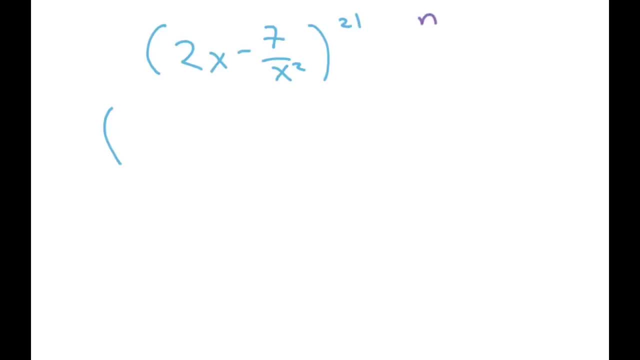 So my N is 21,, so I have 21. choose R, My A is 21.. Okay, So that's 2X, so that's going to be 21 minus R, And my B, as explained before, is negative 7X to the negative 2, because I'm just bringing this up here- to the R, All right. 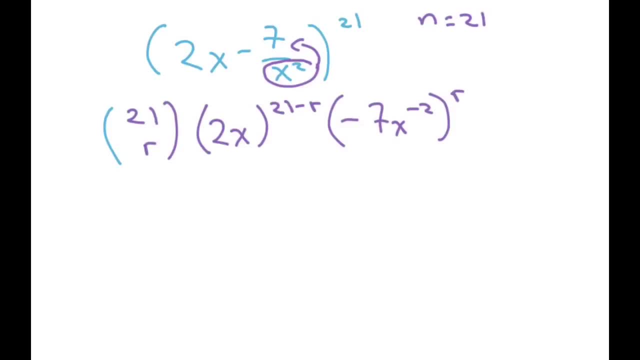 Now, when you first do this it's – you can leave the constants in here, but what I tend to do is just – I want to deal right now with my X's, so I'm just going to pull them out. Okay, So I'm just multiplying what the constant term is. 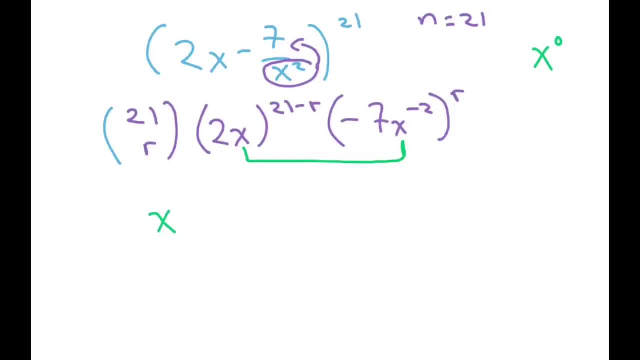 So I have to use this to find R. So I have X to the 21 minus R and then we have X to the negative 2 and multiply that by R And that's supposed to equal X to the 0. Now I'm going to use my product property and combine this. 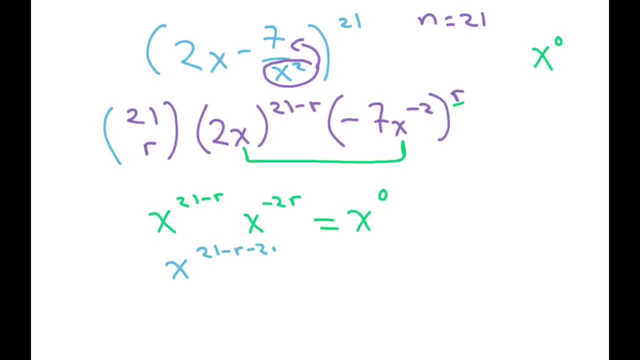 This would be: X, 21 minus R minus 2R equals X to the 0. So I have: X is 21 minus 3.. Okay, So I have: 21 minus 3R equals X to the 0, and since my X is – my bases match – this: 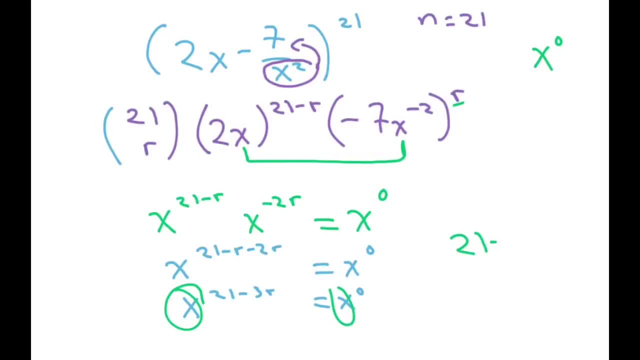 is a base. this is a base – I can just set: 21 minus 3R equals 0 and solve for R, So R equals 7.. Now I'm merely going to plug in my R back into this equation and then solve. 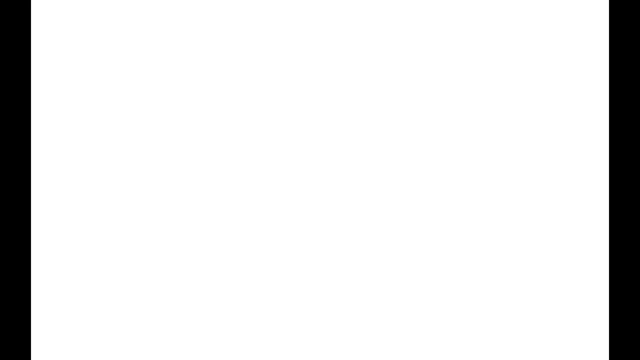 So let me write it again: We have – okay, So I have 21, and now my R is 7.. My A is 2X, and then that's to the M minus R, so that's 21 minus 7.. 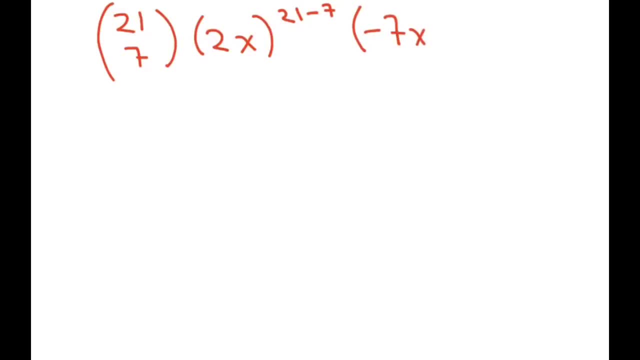 And my B was negative 7X to the negative 2, and then my R now is 7.. So, simplifying this, I can go ahead and – I put this in the calculator And I've got 116, 280.